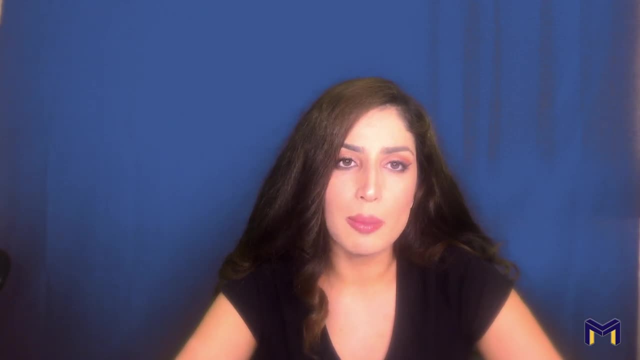 usually covered one or more of these topics, and more advanced topics like planning and control are usually left out. It's my personal opinion that a course in robotics should have all of these topics in tandem, and leaving out one or more of these topics will hinder the learning. In these videos and in 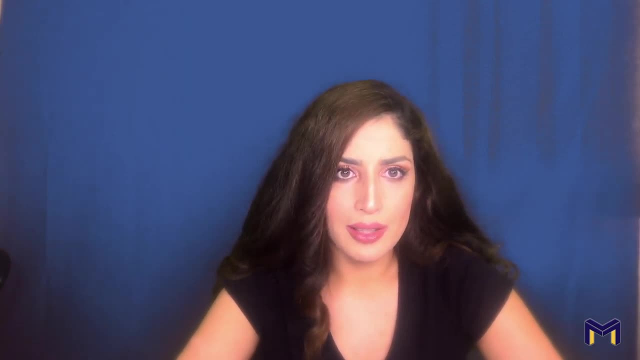 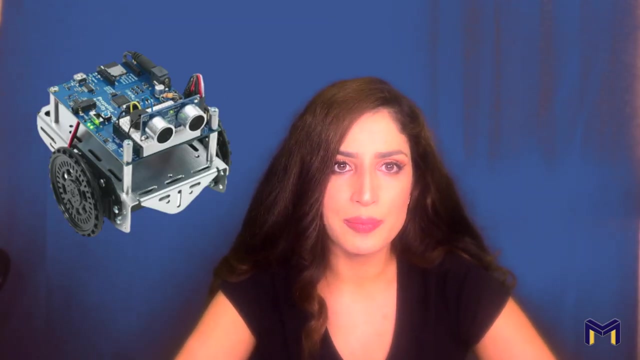 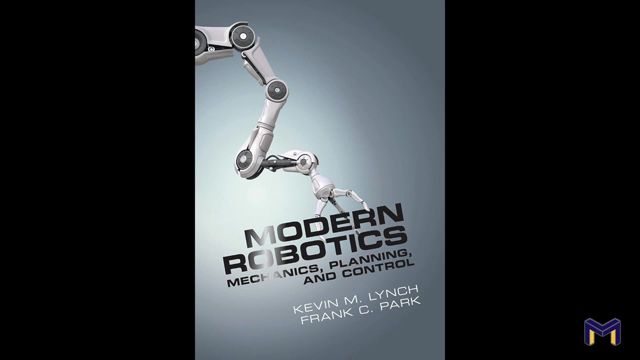 these series. we will use free robot simulators to implement most of the methods discussed. Both robot arms and mobile robots will be covered. Textbooks that are used in the course will be covered. Textbooks that are used in the course are Modern Robotics, Mechanics, Planning and Control by Frank Park and Kevin Lynch. 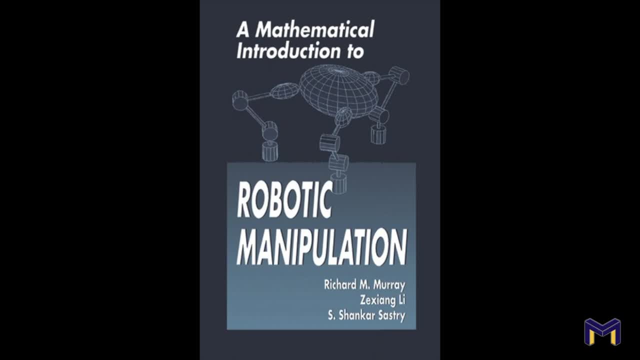 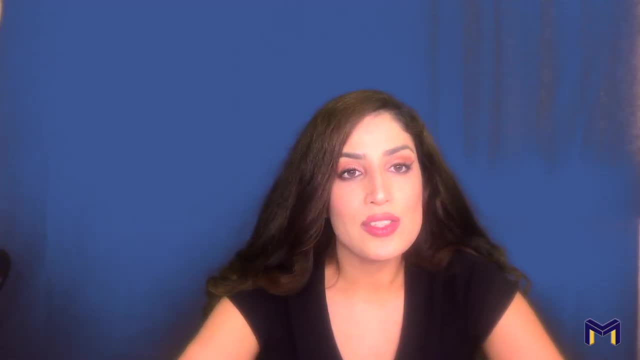 and a Mathematical Introduction to Robotic Manipulation by Murray Lee and Sass Gray. The second book is a little bit advanced and it's usually used in advanced courses, like in graduate school. but I will try my best to make these concepts as easy as possible for you guys to understand. 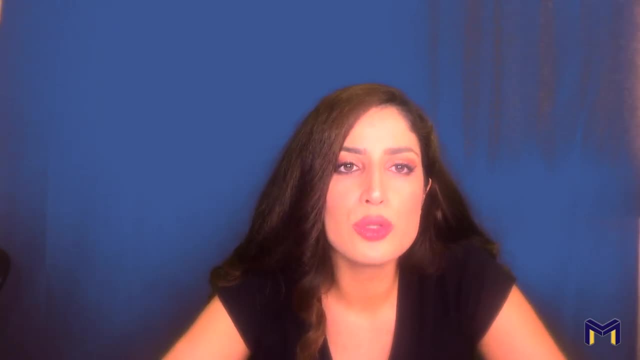 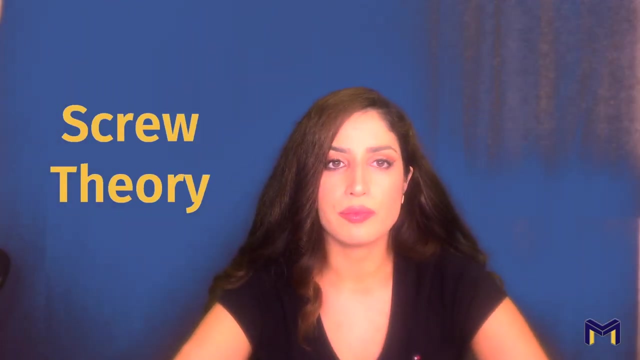 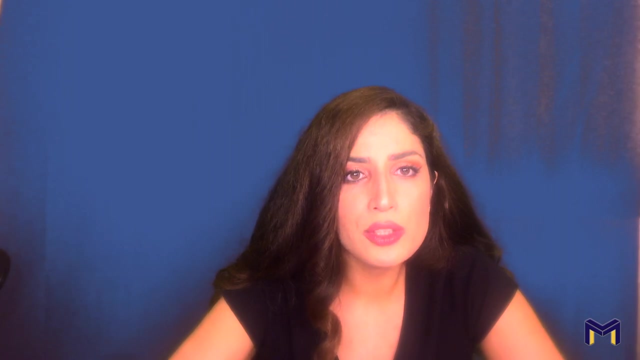 A quick heads up that in these series a modern approach to robotics will be covered. For instance, we will use screw theory to find the kinematics of robots instead of the usual and conventional methods like Denver-Tardy Mark. The modern approach has many advantages that you will see as we go along. All right, if 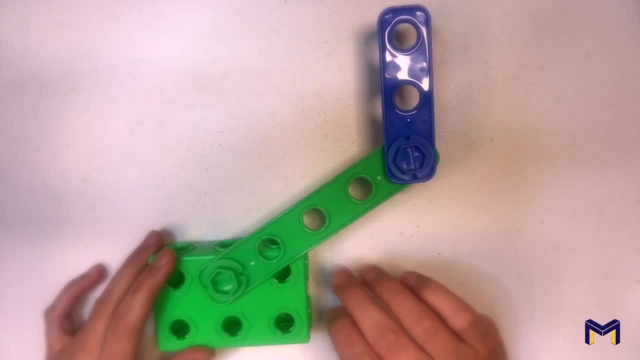 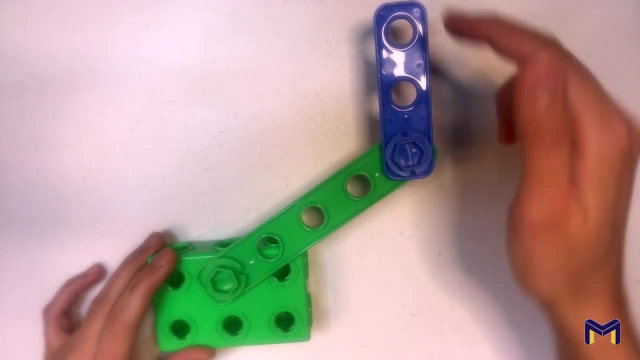 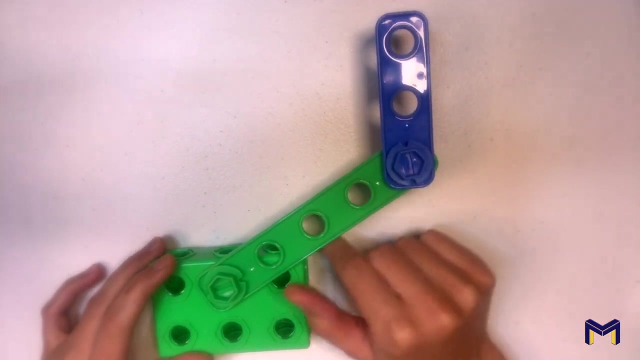 you're ready, let's get started. Okay, a robot consists of links, a joint- and joints. Every joint connects exactly two links. This is my 2DOF planar robot that I'm going to show you guys, these concepts, Actuators which can be for 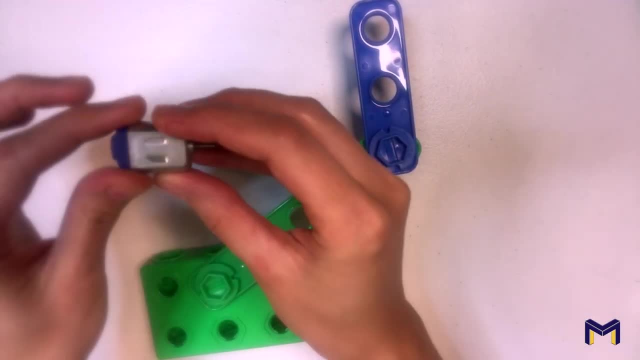 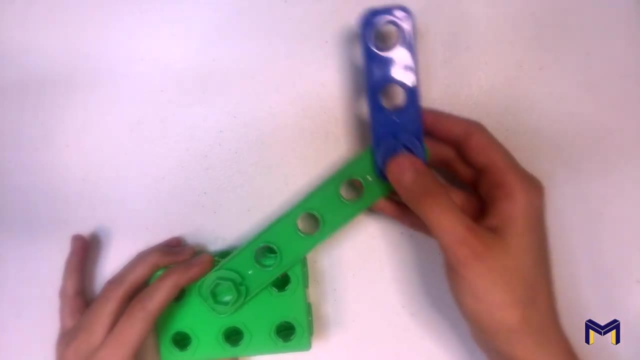 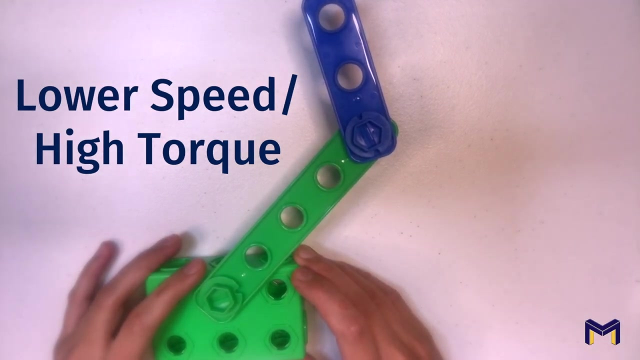 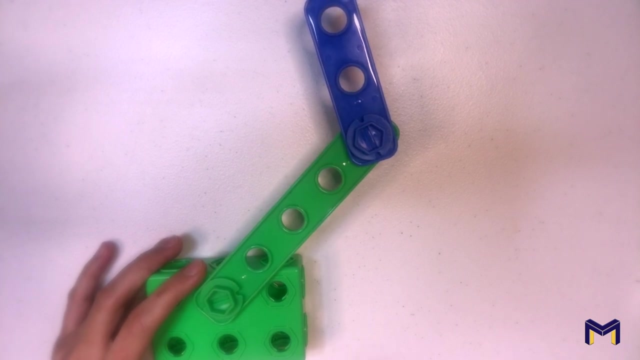 instance, electric motors like the one in my hand. This is the PC motor. It will provide forces and torques that will cause the links to move. It's ideal that the actuators are of lower speed and high torque, but available actuators have speeds in the range of thousands of RPMs and a speed reduction and torque.